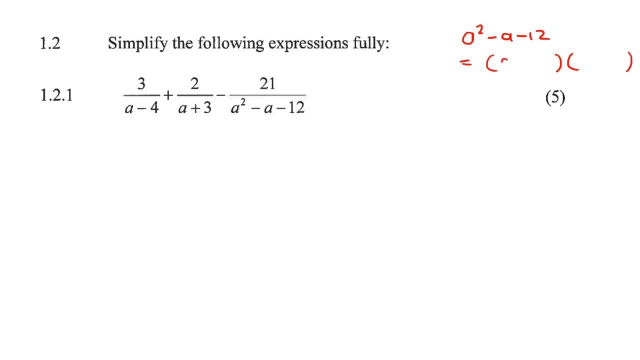 a trinomial, So that would become two different brackets, and then it would be a minus four and a plus three, Because, yeah, if you had to go work this out and multiply those out again, you would see that it gives us that over there. Okay, so now we can just go show them that we've done that. 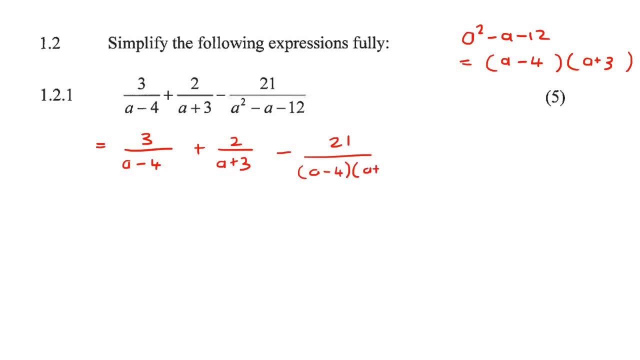 Okay, so we say a minus four and a plus three. So there we have it. All right. Okay, so now we can see that we have a common denominator. That lowest common denominator can just be the a minus four and a plus three. That is what our denominator will be. 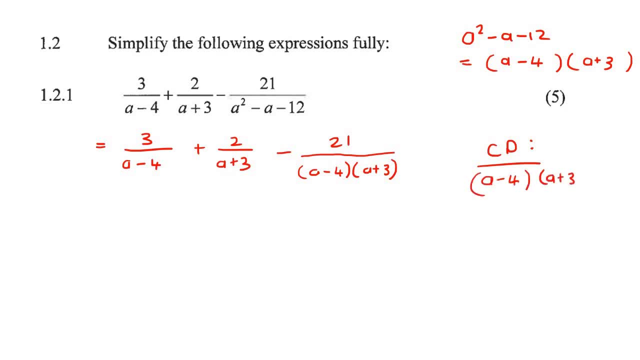 So a minus four. Minus four and a plus three. Okay, so that means that if you look at this one, it still needs what it still needs: a plus three. So we're going to multiply this one with a plus three. And what? 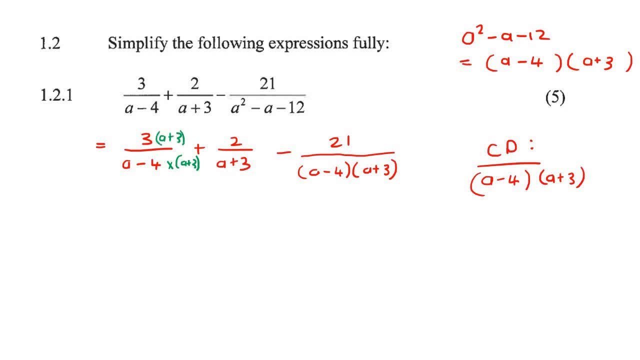 you do at the bottom, you always do at the top. Okay, this one over here still needs to be multiplied with a, a minus four. What you do at the bottom, you always do at the top. And then this one doesn't need anything because it already has both of the elements. 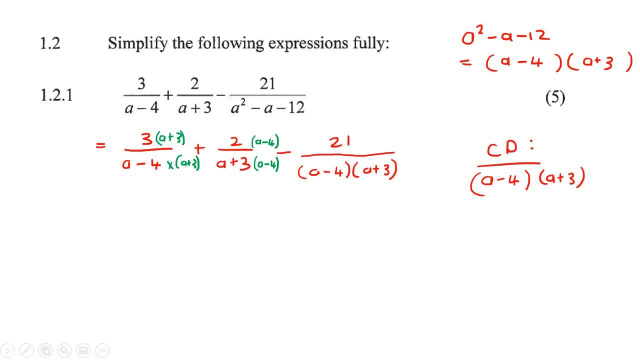 In the periodic table. I'm talking signs here in the lowest common denominator. So in our next step we can then just go and put that bracket up there And then over here we've just gonna put that over there, And then we're going to say plus two. 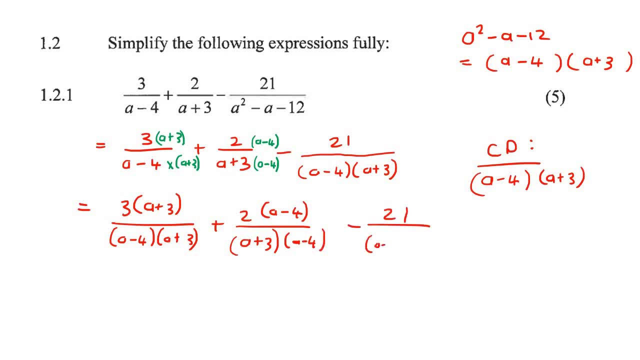 And then like that, and then minus 21.. Okay, there we go. And so what we're doing- we'll do now- is we'll just, we'll just go multiply this, or let me show you, hmm, how could we do this? 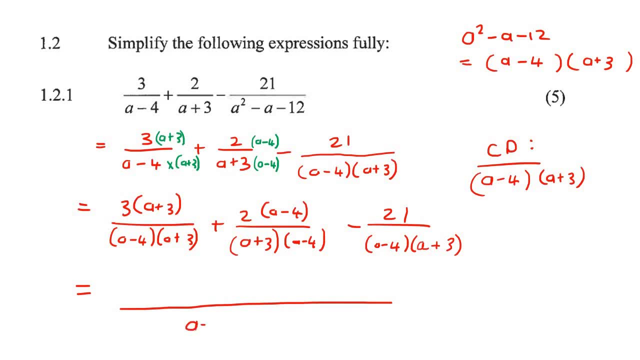 Let me show you a nice way. So we know that the denominators are all the same now. So we can just right the denominator at the bottom like that, And then we can just go for everything in quickly. We don't have to multiply out any brackets just yet. 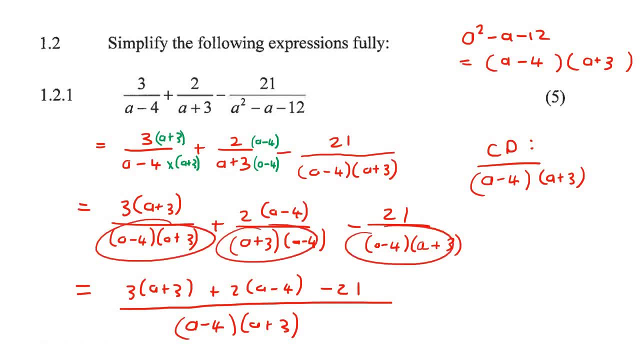 There we go. See what I did. All the denominators are the same, So we can just put all of them over that same denominator. And then now, okay, now in the next step we're just going to go clean up the top part, but we don't. 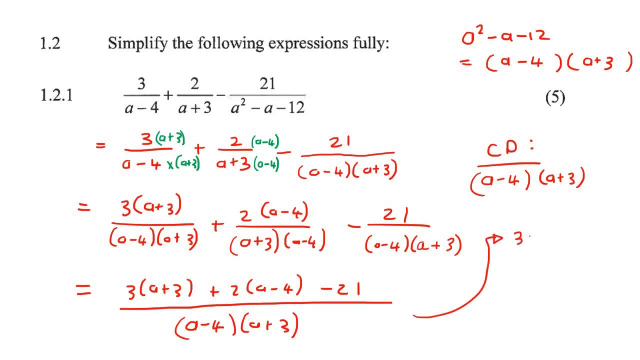 multiply out the bottom part. okay, so at the top we're going to have 3a plus 9 plus 2a minus 8 minus 21 over the denominator which we don't multiply out. that's a minus 4 and a plus 3. 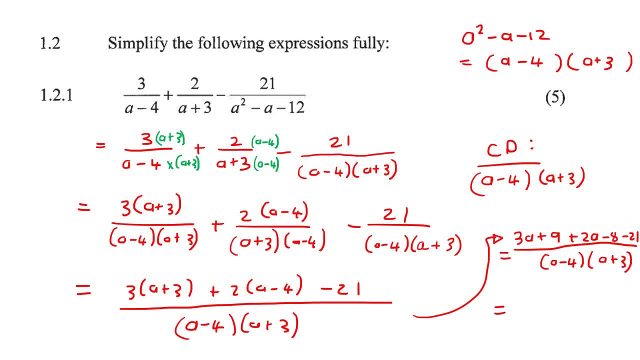 now we can just put like terms together, so for example this 3a and this 2a can become 5a, and then this plus 9 minus 8 is 1, and then 1 minus 21 is minus 20 and then a minus 4. 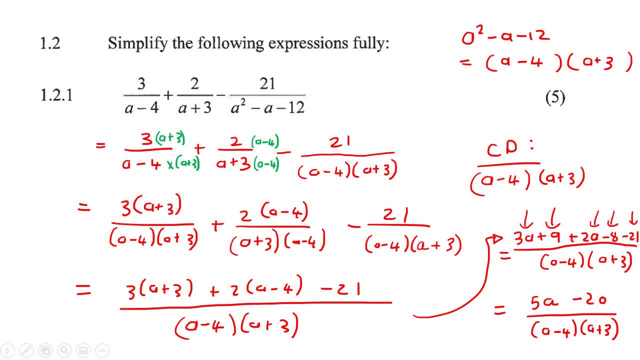 and a plus 3, and then, if you look carefully, we can factorize this part at the top. so sometimes this happens: you, you go ahead, you simplify everything and then it looks, and then you can actually start: um, you can factorize the last part again. okay, so i'm going to quickly erase all of 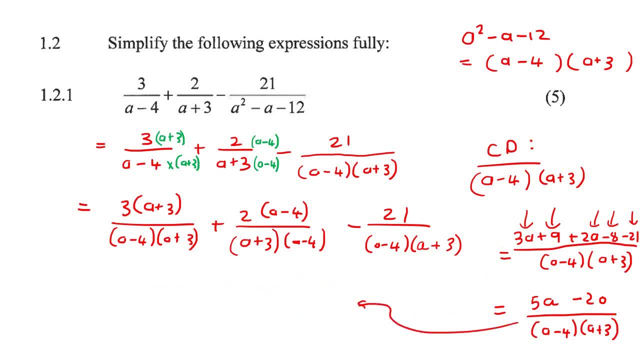 this and go back here. okay, so we'll take out a. so that's going to be, um. you take out a 5 as a common factor at the top and you're left with a minus 4. ah, and then at the bottom, you have a minus. 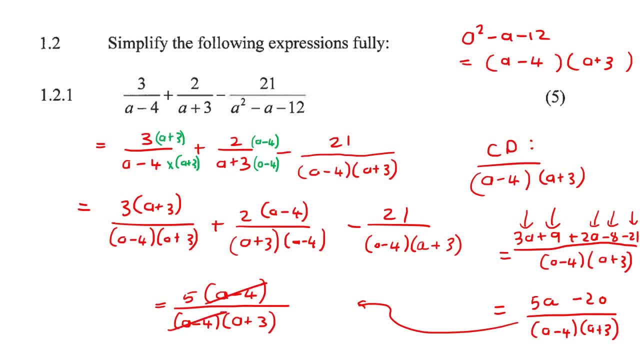 4 and a plus 3, and then these can cancel, and so we are left with a final, final, final answer of 5 over a plus 3. that is the final answer for this question. 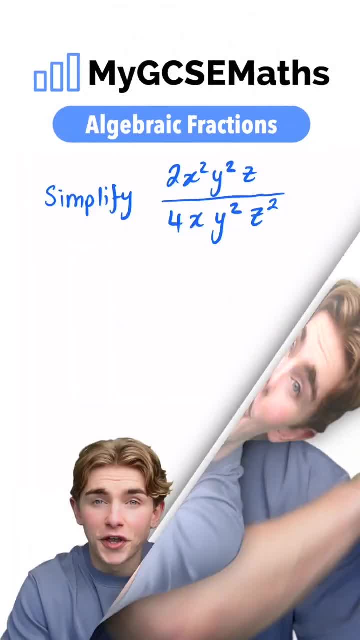 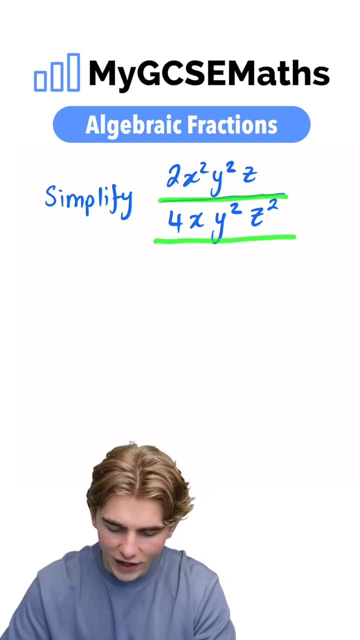 GCSE maths: algebraic fractions in 54 seconds, Let's go. Okay, let's have a look at this. This question asks us to simplify 2x squared y squared z over 4xy squared z squared. How are we going to? 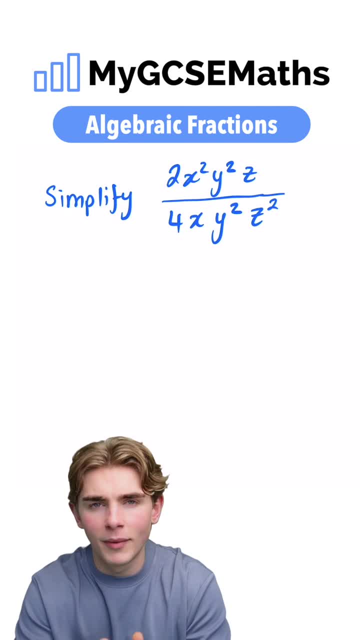 do it Well, we're going to have to divide the numerator and the denominator by any common factors. The difference between this and simplifying a regular fraction is that here those factors are going to be letters instead of numbers, So we can write the numerator as 2.